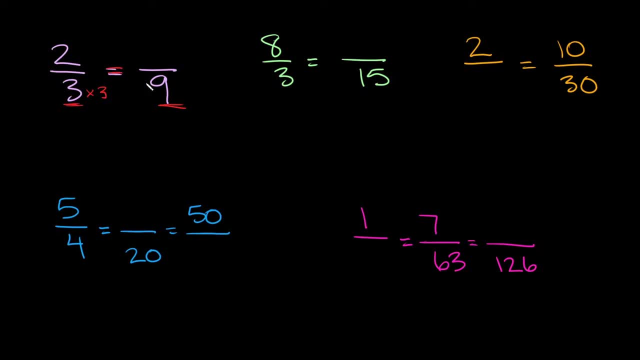 multiply by 3, right, Because 3 times 3 is equal to 9.. Okay, but with equivalent fractions. when you multiply by something on the bottom, you have to multiply by the same thing on top. So if we're going to multiply by 3 down here, we also have to multiply by 3. 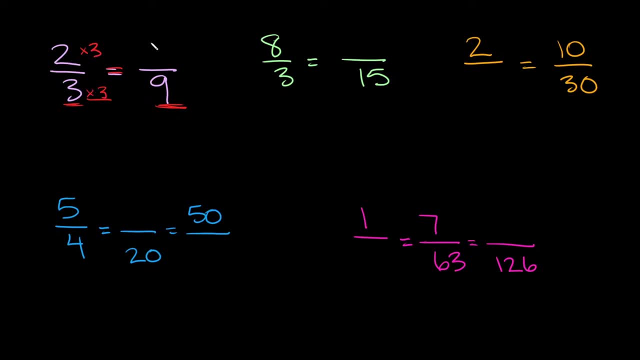 up here. Okay. so what's 2 times 3?? That's equal to 6.. So 2 over 3 or 2 3rds is equivalent to 6 over 9 or 6 9ths. All right, let's do another one. 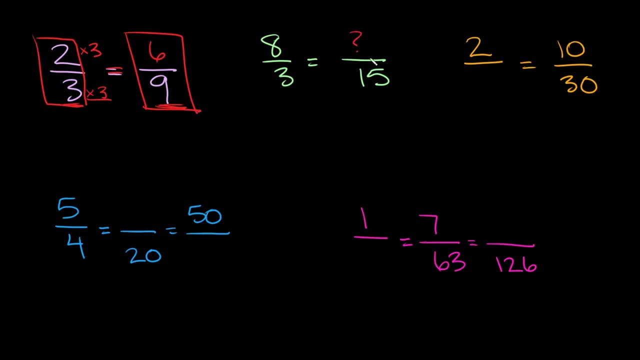 So we have: 8 over 3 is equal to something over 15.. So in this case, we're trying to figure out how we get from 3 to 15.. Okay, well, 3 times 5 is equal to 15, right, So we have to multiply by 5.. 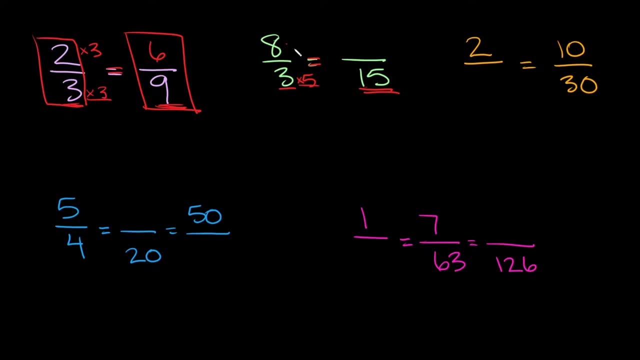 Okay, but remember, if we're going to multiply by 5 at the bottom, we also have to multiply by 5 in the top. So what's 8 times 5?? That's 40. So then we have: 8 over 3 is equal to. 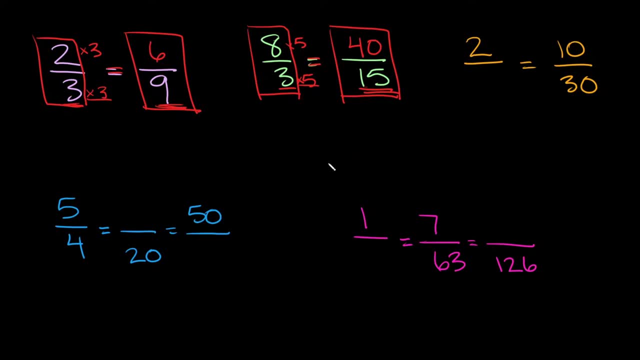 40 over 15.. Okay so these two fractions are equivalent fractions, All right. next example: We have 2 over something is equal to 10 over 30.. Okay so the easier way to solve this problem right here is going from the fraction that you have. 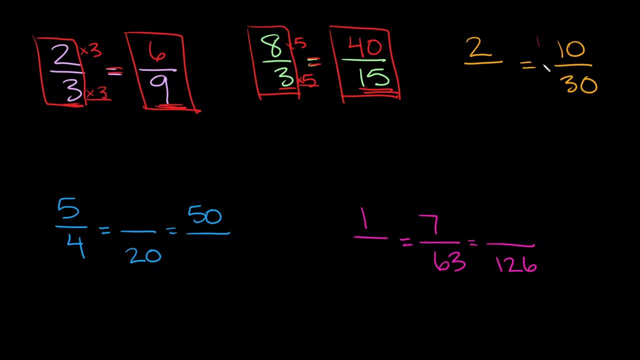 to the fraction that you don't have. So what do I mean by that? So, 10 over 30, we have this fraction, right, It is complete. But this one, 2 over something, this one is incomplete, right? So we want to go from the one that we have, this one, to that one. Okay, so how do we get from 10? 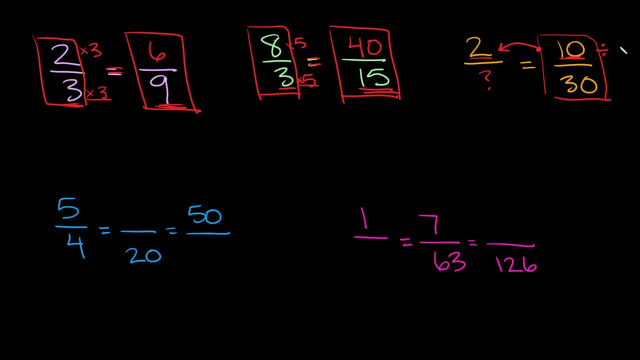 to 2?? Well, we would have to divide by 5, right, 10 divided by 5 is equal to 2.. But remember, whatever you do to the top, you also have to do to the bottom. So if we're going to divide, 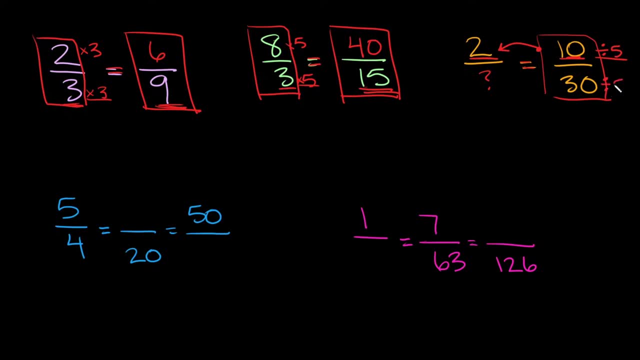 by 5. here we also have to divide by 5 down here. So what is 30 divided by 5?? Well, that would be 5 over 20.. Okay, so 2 over 6 is equal to 10 over 30.. Okay, these are equivalent fractions. 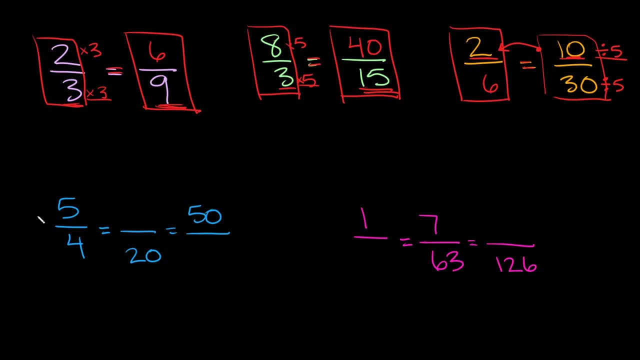 Okay, now let's go to this fraction down here. So remember, we always want to start with the one that we have, the completed one. So here that would be 5 over 4.. Okay, so 5 over 4 is equal to: 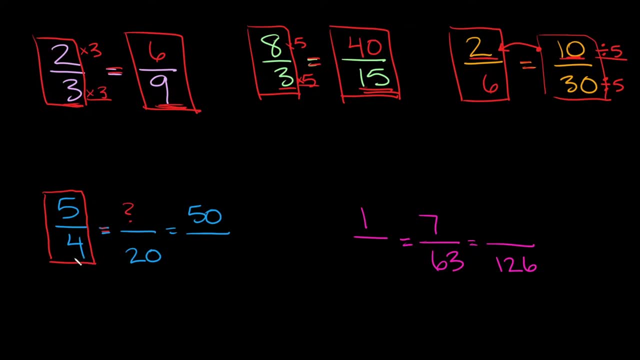 something over 20.. How would we solve this one? Well, in order to get from 4 to 20, you would have to multiply by 5, right? So if we're going to multiply by 5 down here, we also have to multiply. 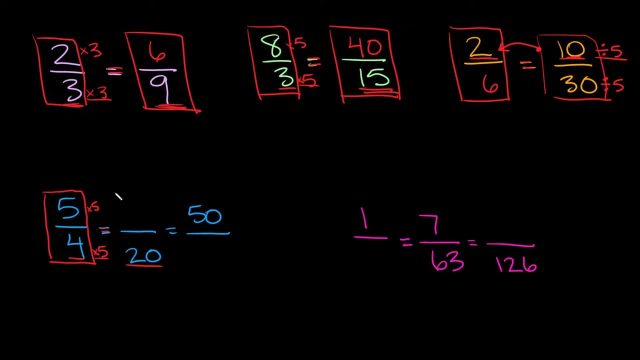 by 5 up here. So what is 5 times 5?? Well, that's just equal to 25.. Okay so, 5 over 4 is equal to 25 over 20.. Okay so, now we have another completed fraction. Okay, so we could either use: 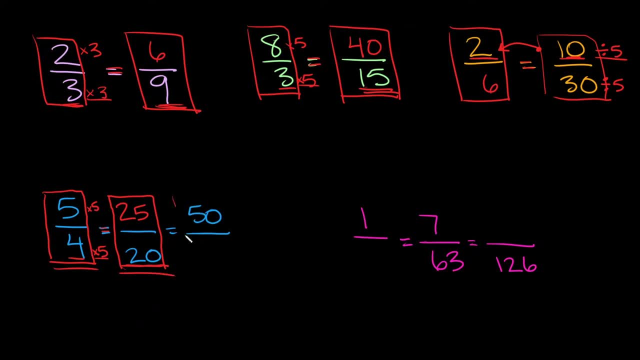 this fraction or this fraction to solve for this last fraction right here. Here's a little tip for your homework or test. Start with the one that you're given, because if you use this one and you made a mistake on it, well, when you use it, you're also going to get a mistake on this one, right? 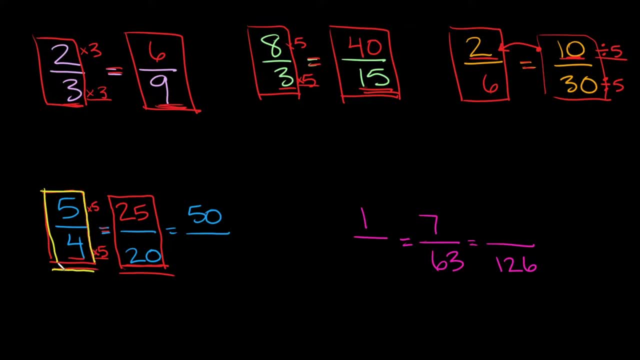 But this first one, this original one, was given to us, so we know it's correct. So let's just use this one. Okay, so we have: 5 over 4 is equal to 50 over something. So how do you get from 5 to 50?? 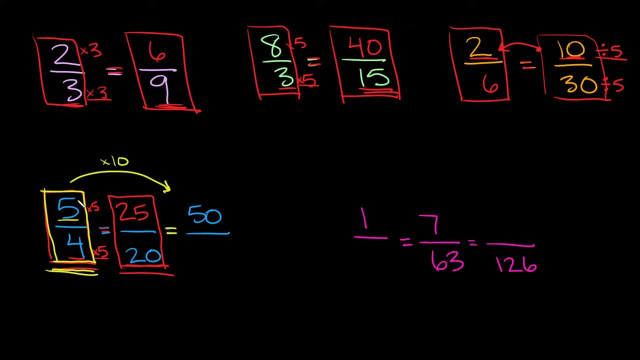 Well, you have to multiply by by 10. it looks like, right, 5 times 10 is equal to 50.. Okay, so if we're going to multiply by 10 up here, we also have to multiply by 10 down here. Okay, so, what's 4 times 10?? That's 40.. 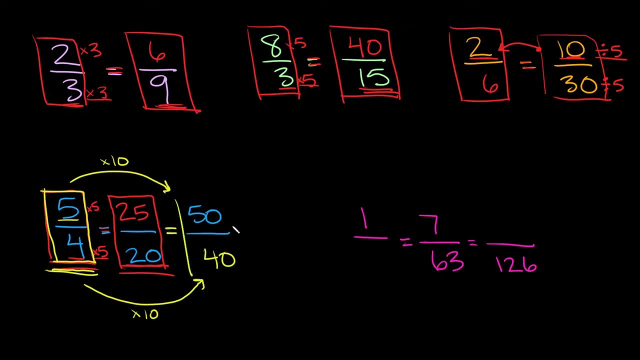 Okay, so 5 over 4 and 50 over 40 are equivalent fractions. Okay, now let's do this last one. So the one that we are given is this one right: 7 over 63.. So how do we get from 7 to 1?? Well, we would have to. 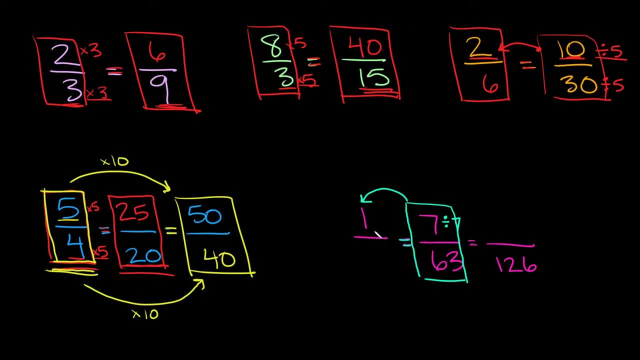 divide by 7, right, 7 divided by 7 is equal to 1.. So that means we're going to have to also divide by 7 on the bottom, All right. so what's 63 divided by 7? Well, that's just equal to 9.. 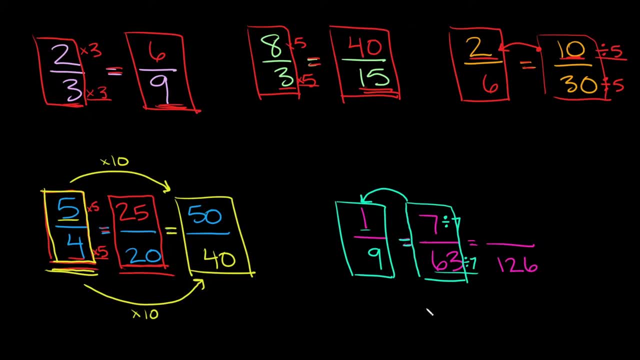 Okay, so 1 over 9 and 7 over 63 are equivalent fractions. Okay, so we just have this last one, So we're going to have to figure out. So, again, I'm going to start with the one that I was given. So. 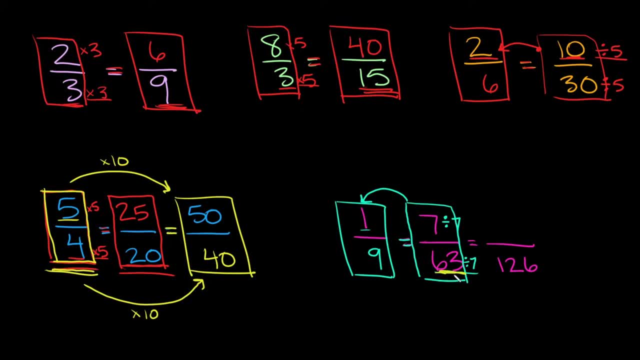 7 over 63.. How do I get from 63 to 126?? Well, let's see 63,. that's pretty close to 60, right? And if I multiply it by 2, or in other words, if I double it, that would be 120, right. 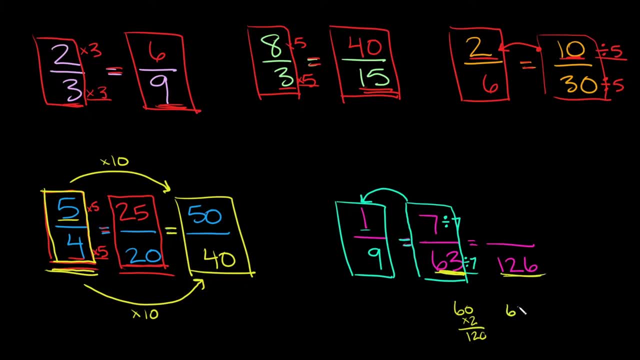 Which is pretty close to 126.. So I think 63 times 2 might be 126.. Let's see, 3 times 2 is 6, and then 2 times 6 is 126.. Okay, so that checks out right. So to get from 63 to 126,. 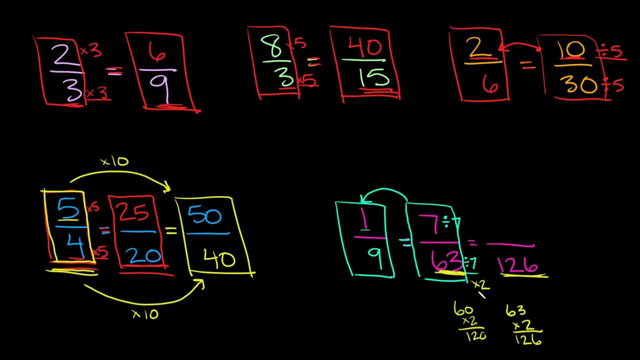 we have to multiply by 2, right, But again, if I'm going to do it at the bottom, I have to multiply by 2 at the top. So what's 7 times 2? That would be 14.. Okay, so 7 over 63 is equal to. 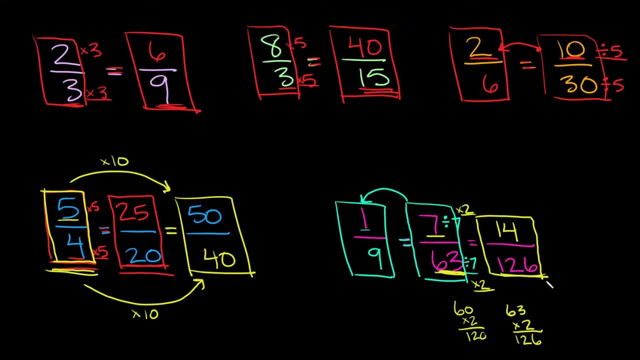 14 over 126.. All right, guys, so that's how you find the missing number of equivalent fractions. I hope the examples were helpful. If they were definitely, leave a thumbs up down below, And if you still got questions, leave them in the comment section below and I'll do my best to try and help you out. 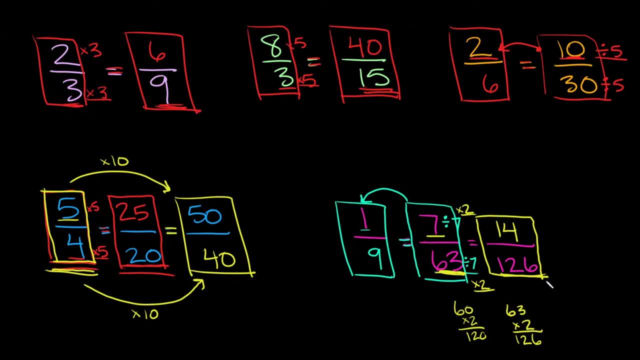 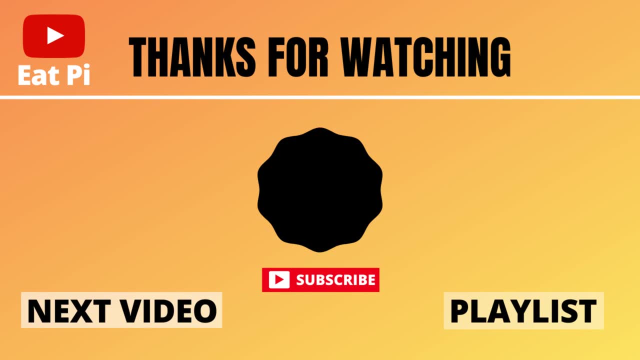 Also, there's a playlist attached at the end of the video, So if there's any other topics you need help with, definitely check that out and I'll see you there. Thanks for watching and I'll see you in the next one.